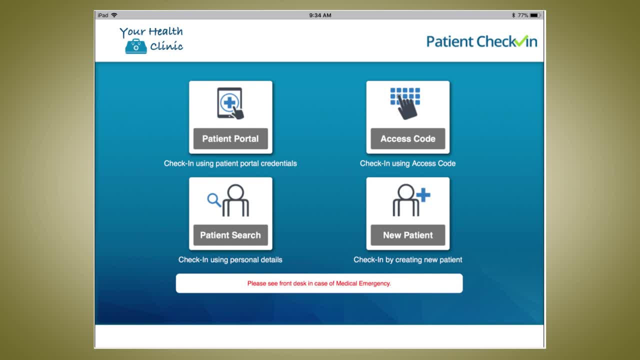 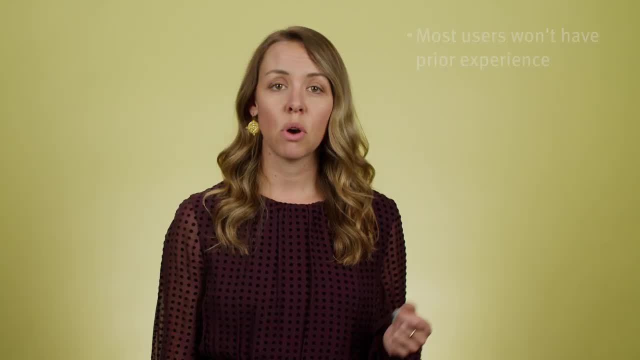 tablet application used by patients of a health clinic so that when they arrive for their appointment, they can check in and update any personal information that's on file. Most users probably wouldn't have much, if any, prior experience with a type of tool like this. 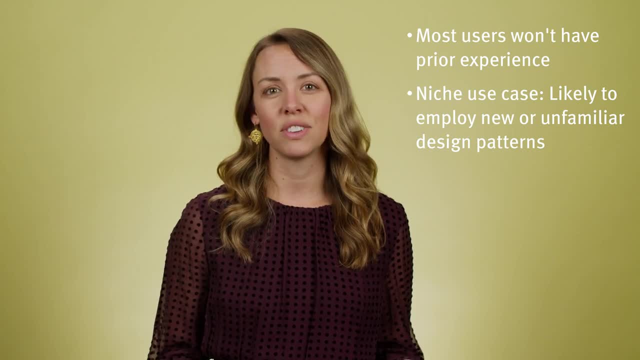 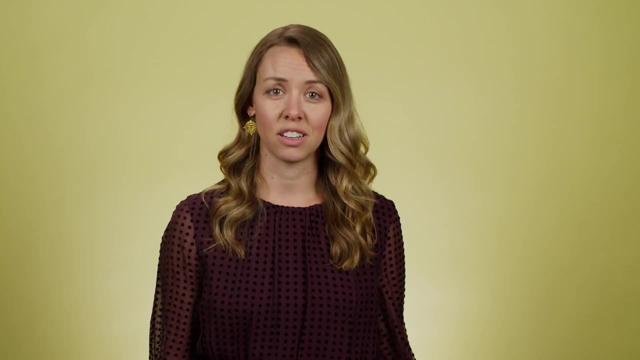 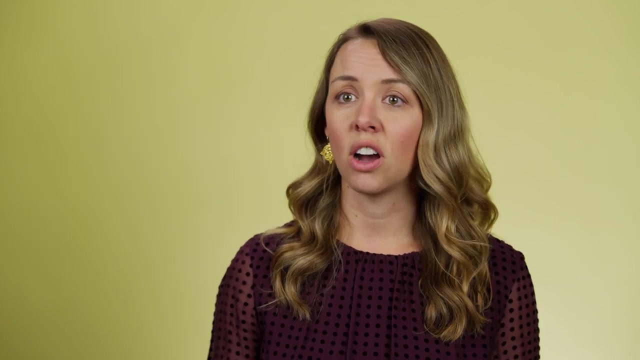 And because it has a very niche use case, the interface itself is likely to employ new or unfamiliar design patterns. These factors are what make it a good candidate for a cognitive walkthrough assessment. On the flip side, doing a cognitive walkthrough to assess something like an e-commerce checkout- 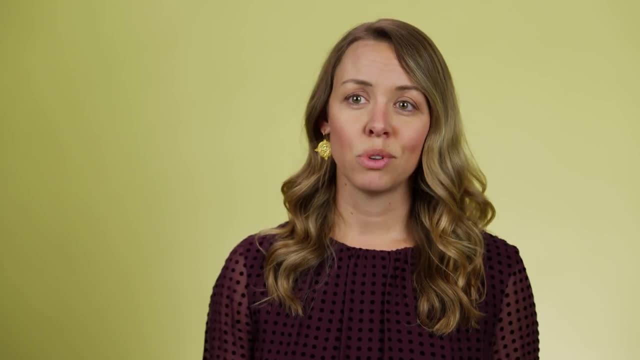 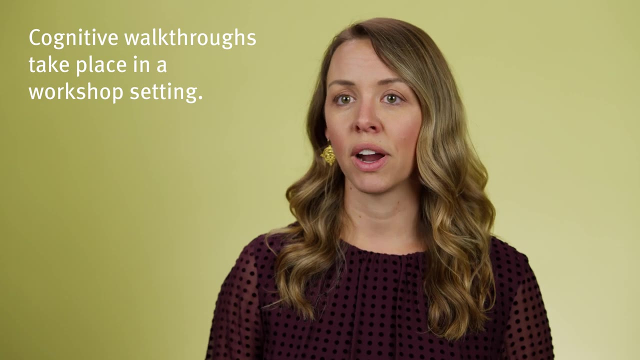 flow probably wouldn't be necessary, since most people are pretty familiar with these types of experiences. Cognitive walkthroughs take place in a workshop setting where a cross-functional team of reviewers can work together to assess the design of the interface. The interface is a kind of platform where the reviewer's team of reviewers come together and literally. 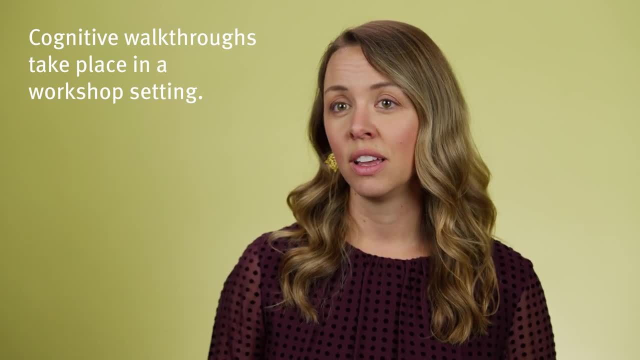 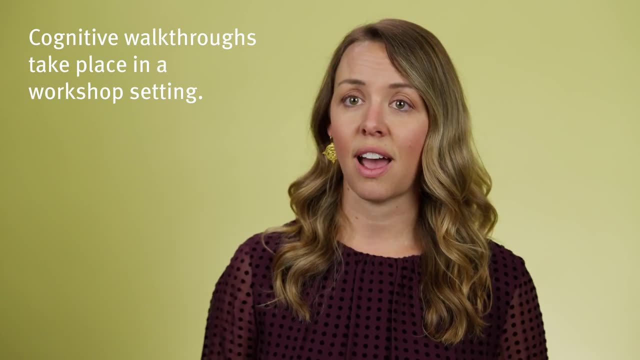 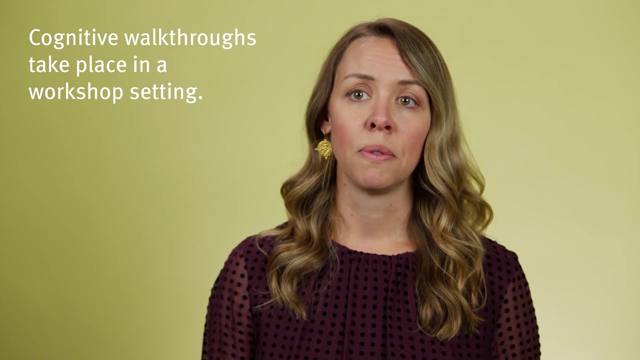 walk through each step of a user flow And collectively they answer a set of prescribed questions for analysis. The goal is to identify aspects of the interface that might be challenging for new users. Walkthrough reviewers might include people of various UX specialty product. 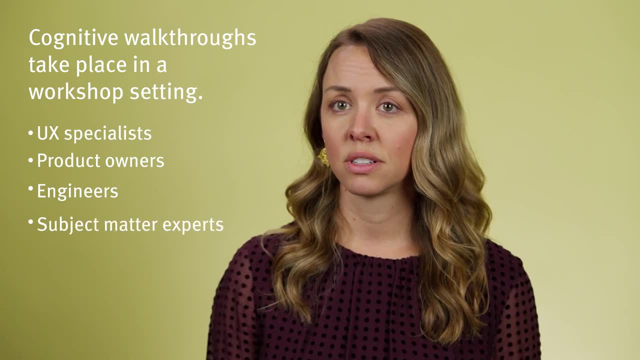 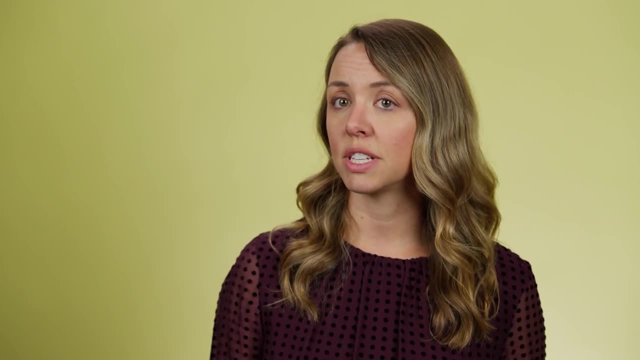 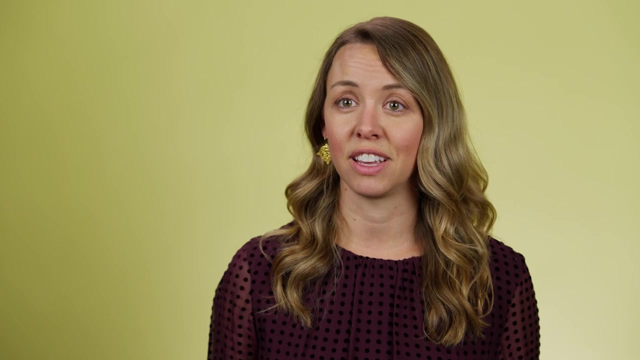 owners, engineers or subject matter experts. A facilitator leads the group of evaluators through the task. A reviewer should be able to identify the elements of the interface task flow, while the evaluators offer their interpretation of how a particular type of user might perceive the interface and thus how they might behave in a given situation. 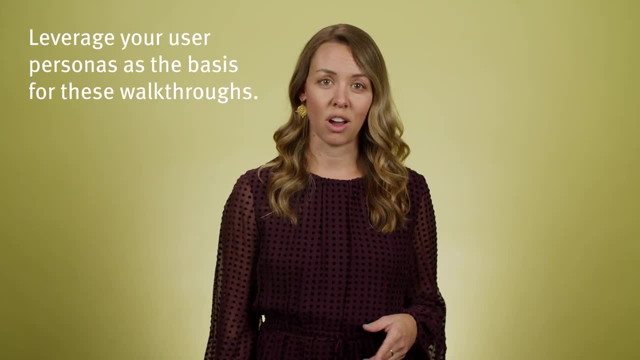 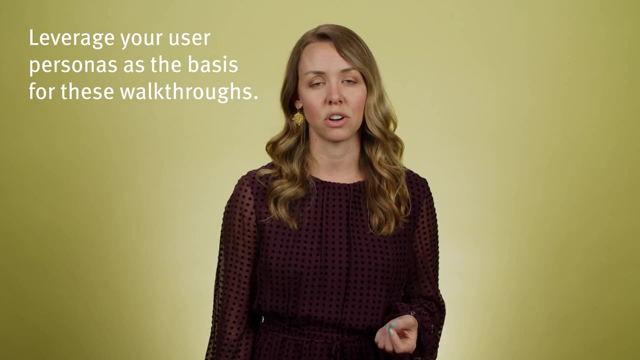 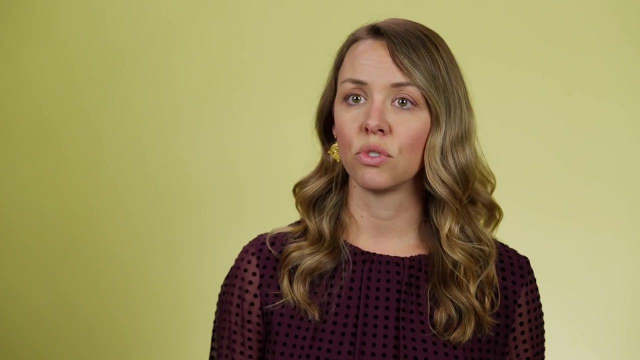 It's a great idea to leverage your user personas as the basis for these walkthroughs, because they'll help you to get everyone on the same page around the context and mindsets of the users for which they're evaluating Now. during the actual evaluation of a given task, the facilitator moves through the interface. 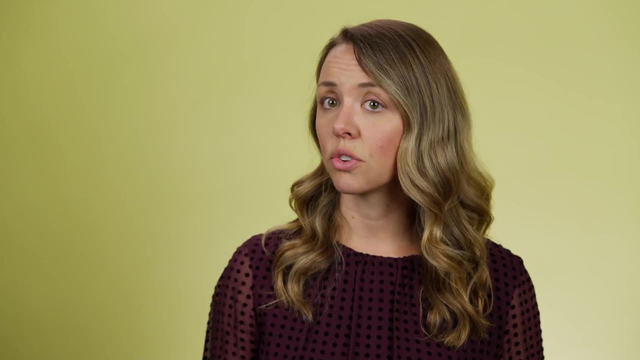 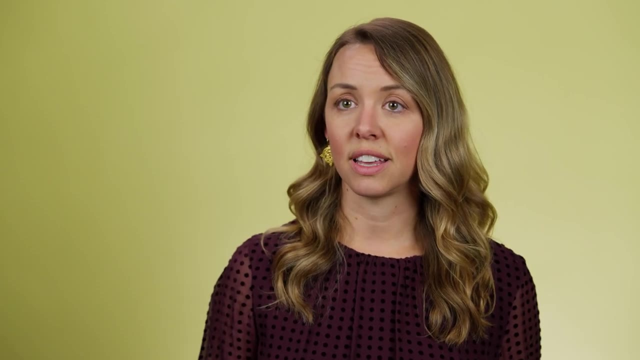 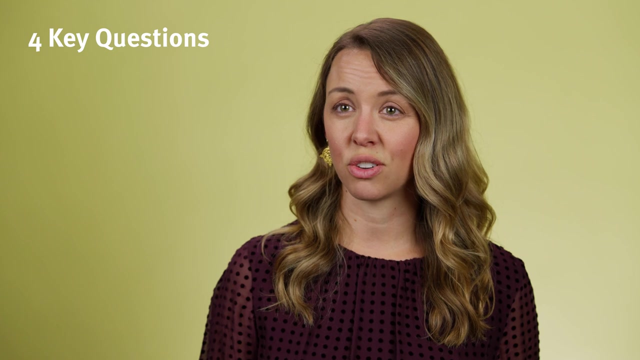 and stops at each new screen or, if not a new screen, each new discrete step in the interaction flow. Then, to establish whether the user is likely to succeed or fail, at each step, the evaluators discuss four key questions designed to uncover potential fail points. 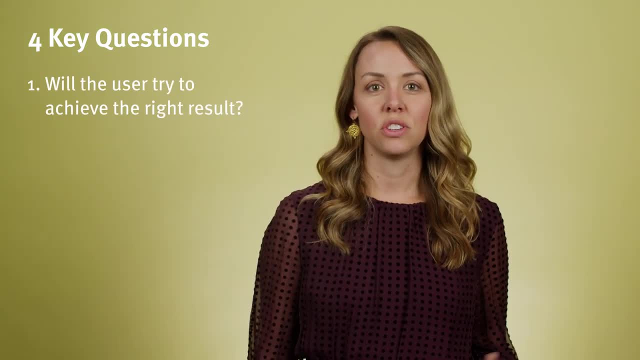 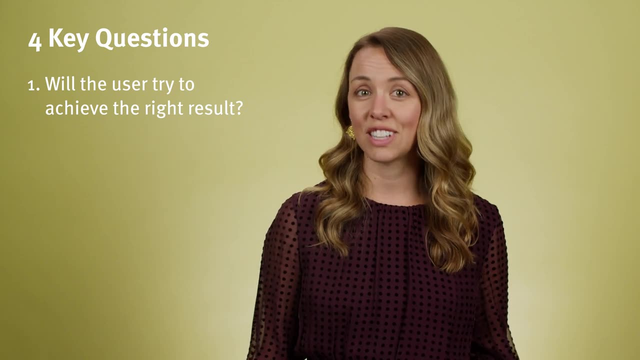 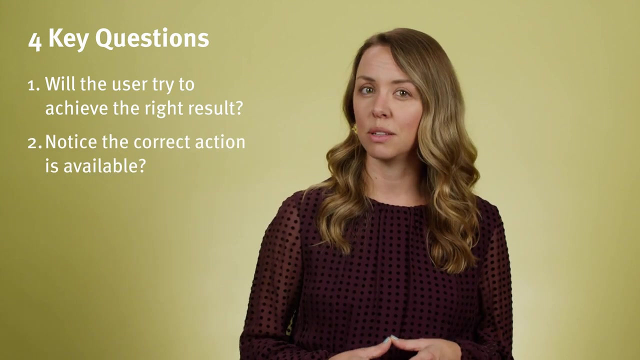 The first question for analysis is: will the user try to achieve the right result? In other words, would the user understand that the action or necessary next step is necessary to reach their larger goal? Prompt number two asks: will the user notice that the correct action is available?